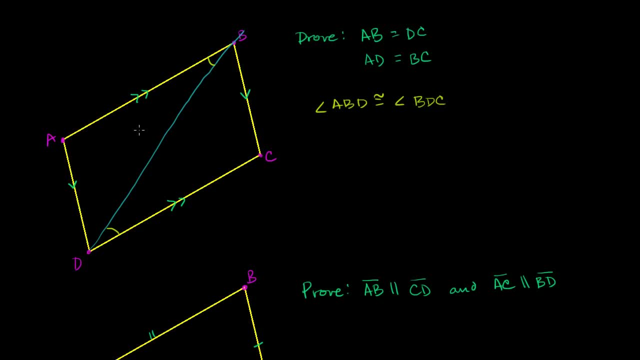 you could view it as a transversal of these two parallel lines, of the other pair of parallel lines, AD and BC. And if you look at it that way, then you immediately see that angle DBC, right over here, is going to be congruent to angle ADB for the exact same reason. 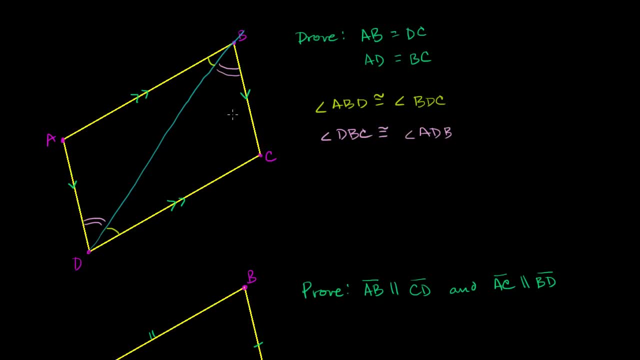 They are alternate interior angles of a transversal intersecting these two parallel lines. So I could write this: this is alternate interior angles. interior angles are congruent when you have a transversal intersecting two parallel lines. And we also see that both of these triangles- triangle ADB. 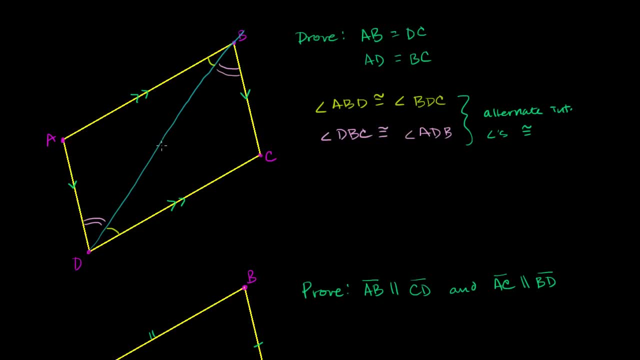 and triangle CDB both share this side. over here. It's obviously equal to itself. Now, why is this useful? Well, you might realize that we've just shown that both of these triangles they have this pink angle, then they have this side in common, and then they. 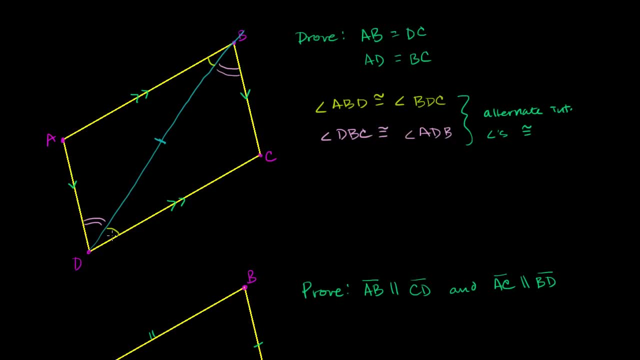 have the green angle, Pink angle side in common and then the green angle. So we've just shown by angle side angle that these two triangles are congruent. So let me write this down: We have shown that triangle. I'll. 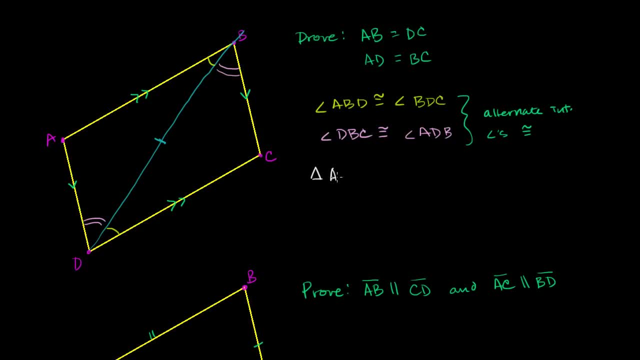 go from non-labeled to pink to green ADB is congruent to triangle. non-labeled to pink to green CCBD And this comes out of angle side angle congruency. So this is from angle side angle congruency. 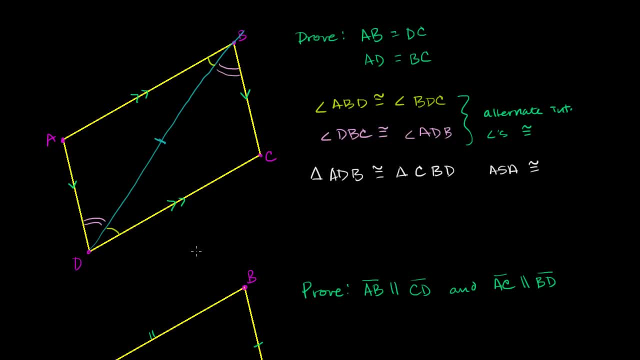 Well, what does that do for us? Well, if two triangles are congruent, then all of the corresponding features of the two triangles are going to be congruent. In particular, side DC corresponds to side BA, So side DC on this bottom triangle. 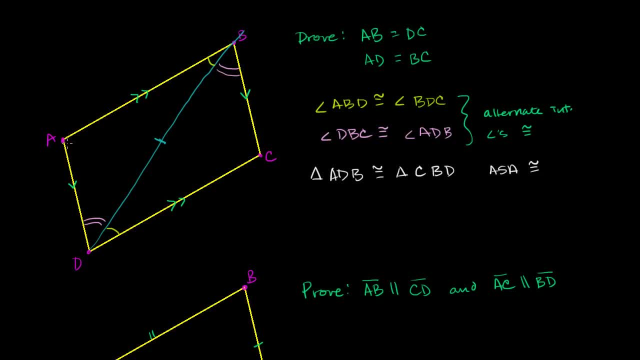 corresponds to side BA on that top triangle. So they need to be congruent. So DC is going to be equal to BA, And that's because they are corresponding sides of congruent triangles. So this is going to be equal to that And by that exact same logic, AD corresponds. 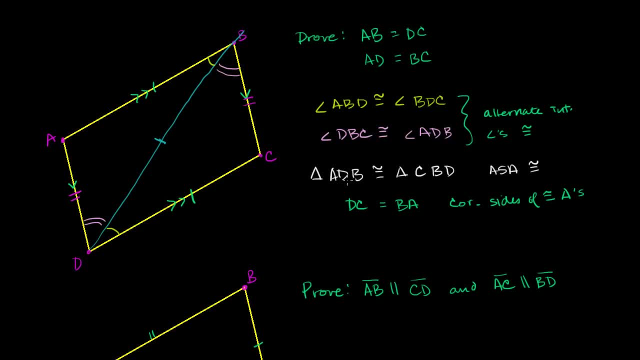 to CB and, for the exact same reason, corresponding sides of congruent triangles. And then we're done, We've proven that opposite sides are congruent. Now let's go the other way. Let's say that we have some type of a quadrilateral. 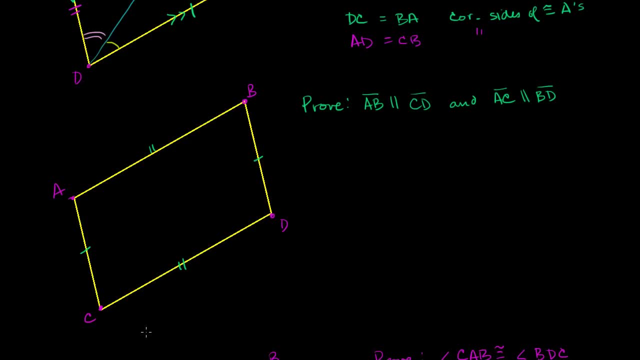 and we know that the opposite sides are congruent. Can we prove to ourselves that this is a parallelogram? Well, it's kind of the same. It's proof in reverse. So let's draw a diagonal here, since we know a lot about triangles. 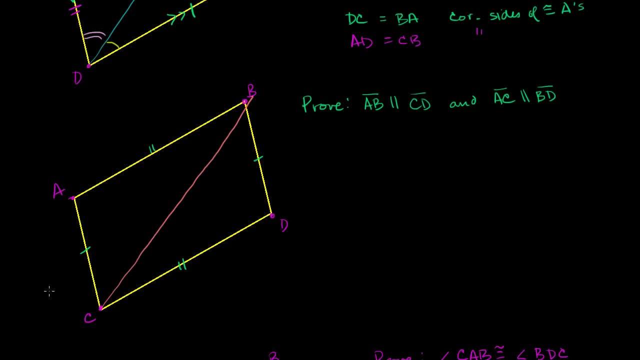 So let me draw. There we go. That's the hardest part. Let's see, Draw it. That's pretty good, All right. So we obviously know that CB is going to be equal to itself, So I'll draw it like that. 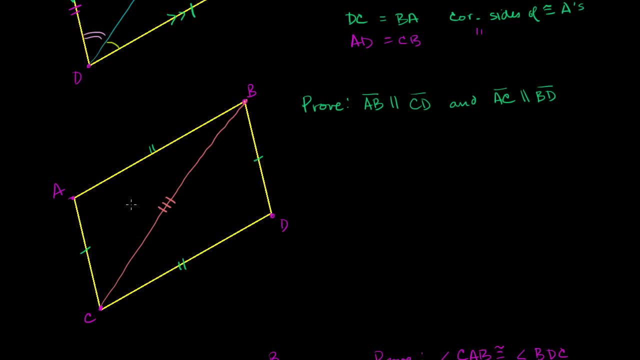 Obviously, because it's the same line. And then we have something interesting: We've split this quadrilateral into two triangles- triangle ACB and triangle DBC- And notice all three sides of these two triangles are equal to each other. So we know by side side side that they are congruent. 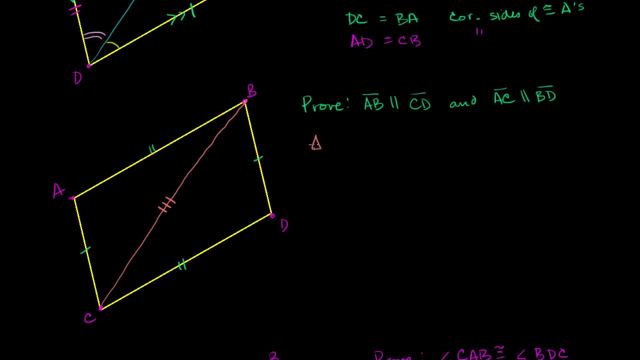 So we know that triangle A and we're starting at A and then I'm going to the one hash side. So ACB is congruent to triangle DBC, And this is by side side side, side side side congruency. 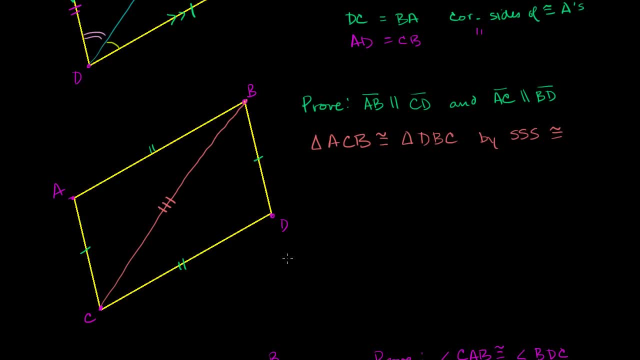 Well, what does that do for us? Well, it tells us that all of the corresponding angles are going to be congruent. So, for example, ABC, angle ABC is going to be. so let me mark that angle ABC is going to be congruent. 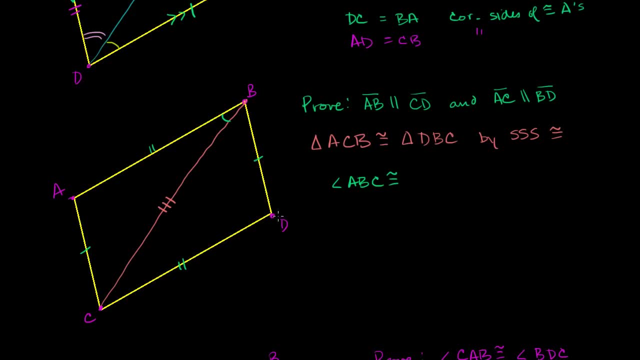 And you can say: ABC is going to be congruent to DBC. OK, And you can say: by you can say corresponding angles congruent of congruent triangles. I'm just using some shorthand here to save some time. So ABC is going to be congruent to DCB. 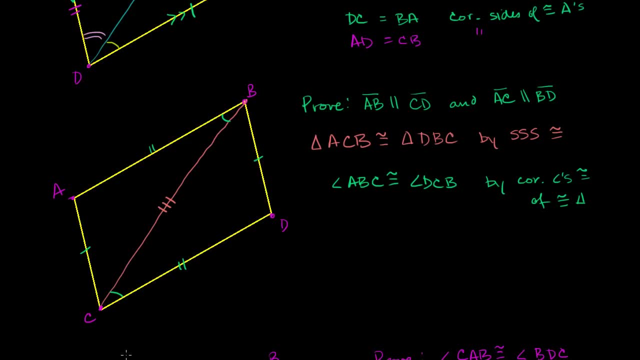 So these two angles are going to be congruent. Well, this is interesting because here you have a line and it's intersecting AB and CD, And we clearly see that these things that could be alternate angles, alternate interior angles, are congruent. 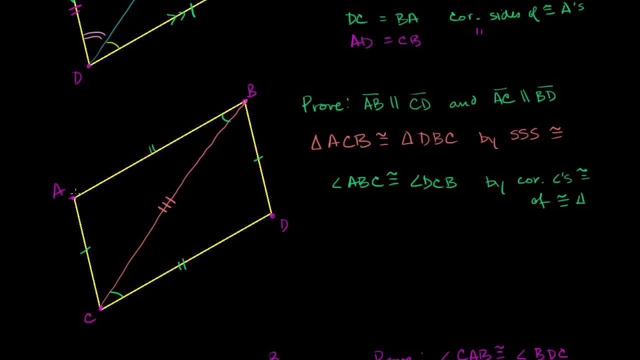 And because we have these congruent alternate interior angles, we know that AB must be parallel to CD. So this must be parallel to that. So we know that AB is parallel to CD by alternate interior angles of a transversal intersecting parallel lines. 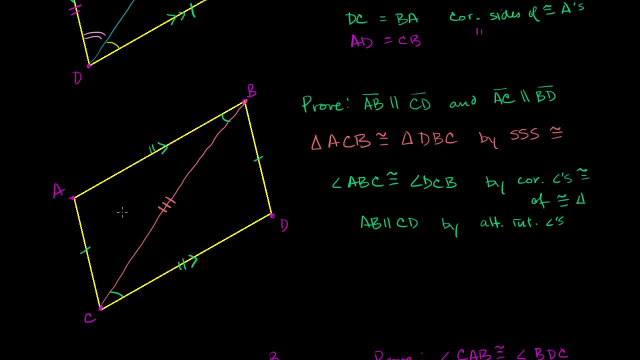 Now we can use that exact same logic. We also know that angle. let me get this right: angle ACB is congruent to angle DBC And we know that by corresponding angles, congruent of congruent triangles. So we're just saying that this angle is equal to. 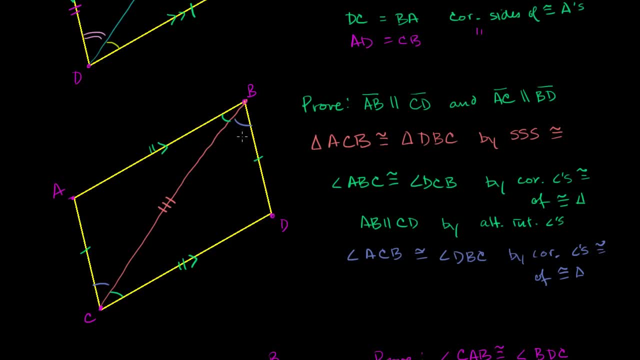 let's say ACB by alternate interior angles. Well, once again these could be alternate interior angles. They look like they could be. This is a transversal And here's two lines here which we're not sure whether they're parallel. 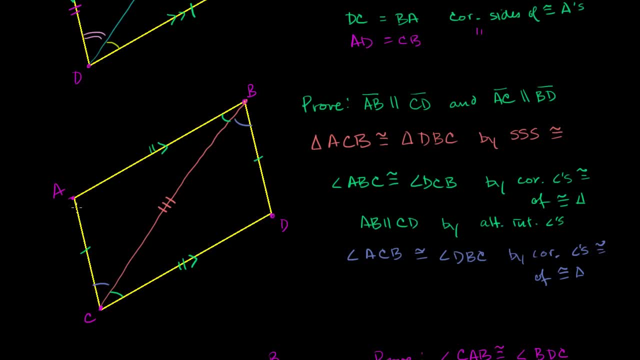 But because the alternate interior angles are congruent, we know that they are parallel. So this is parallel to that. So we know that AC is parallel to BD by alternate interior angles, And we're done. So what we've done is it's interesting. 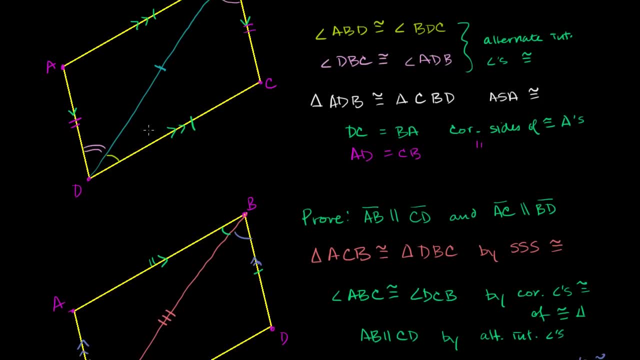 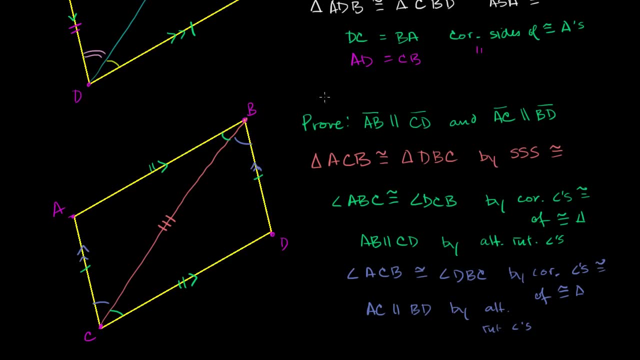 We've shown, if you have a parallelogram, opposite sides have the same length, And if opposite sides have the same length, then you have a parallelogram, And so we've actually proven it in both directions, And so we can actually make what you call an if, and only if.